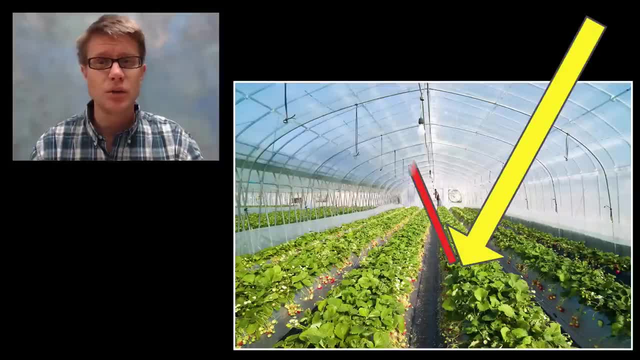 being reflected. Now let's look at light that is then converted into infrared radiation or heat. What happens to that? Well, when it hits the glass, some of it is going to be lost as heat to the environment, but some of it is refracted or bent back into the greenhouse, And that gets bounced around. 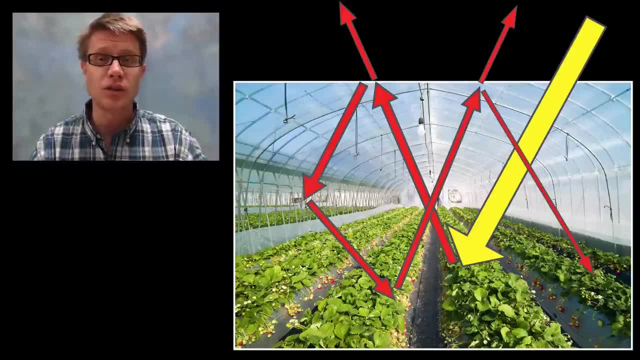 lose some of it, And so that heat is going to stay inside the greenhouse effect. Now, if we can limit convection or the movement of the air, then we can keep all that heat inside a greenhouse. It works a little bit different in our atmosphere, And so how does? 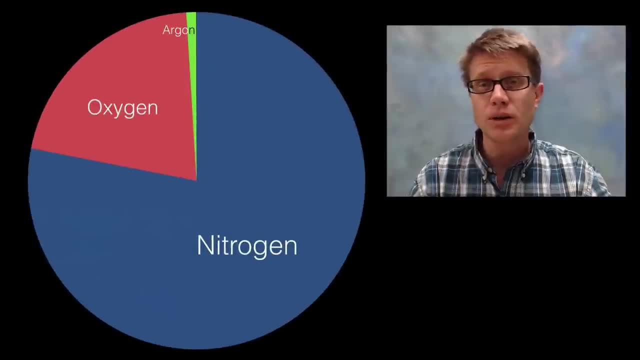 our atmosphere keep heat close to it. Well, let's look at what the atmosphere is made up of. It's mostly nitrogen, like 78% of it. We've got about 21% oxygen. We've got around 1% argon, And then there's this really tiny little black band right here And that's going. 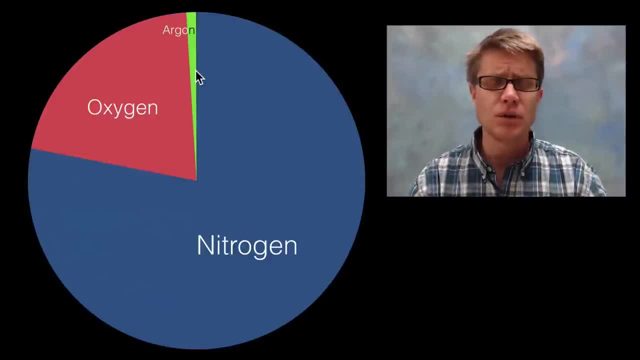 to represent everything else. Now, water can vary, And so we could have up to 4% of the atmosphere dealing with water, But we still have this really faint line here that you can't even see. And so what's inside there? Well, a lot of the greenhouse gases are inside. 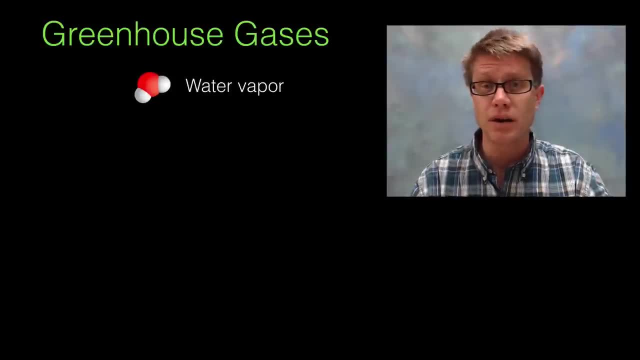 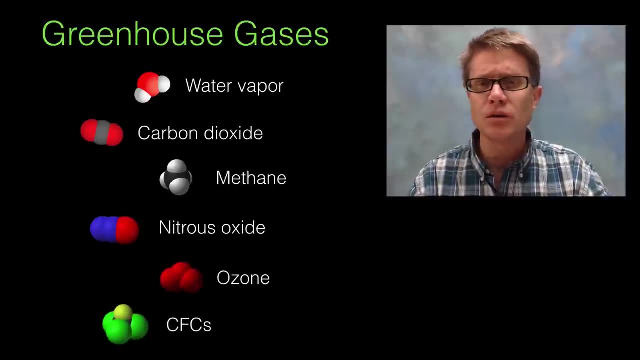 there. And so what does that list contain? It contains water vapor, But it also contains carbon dioxide, methane, nitrous oxide, ozone- which is actually really important- And then close it to the atmosphere. And then what's inside of that? Well, it contains hydrogen. 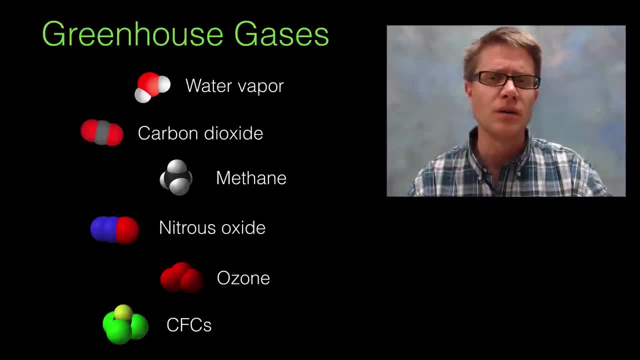 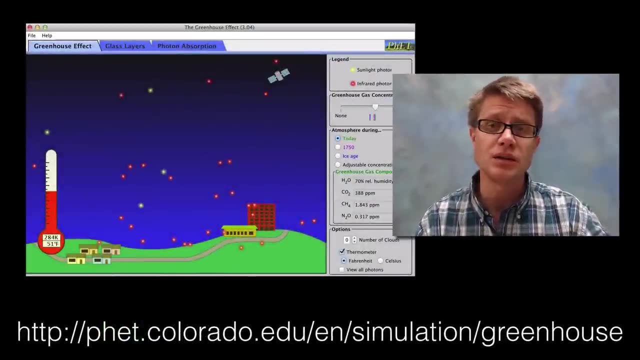 of fluorocarbons And a lot of those are produced by humans, And these are all greenhouse gases, And so how do they hold heat in? Well, I'm going to use a simulation to show you this. This is a PHET simulation, And so I'll put a link in the video description down below. 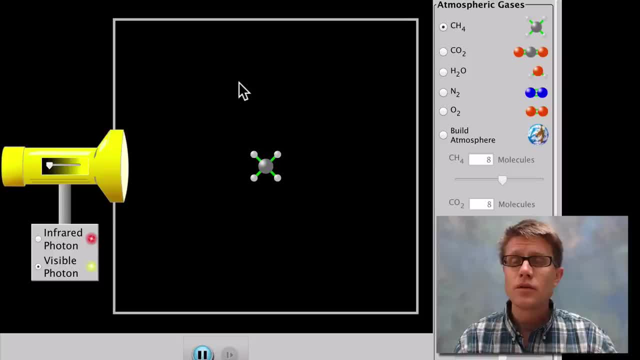 I would encourage you to go there and check it out, But let's take a look at that. First thing you should look at is how visible photons and infrared photons interact with the gases that we're going to find in the atmosphere, And so in this simulation, we've got methane. 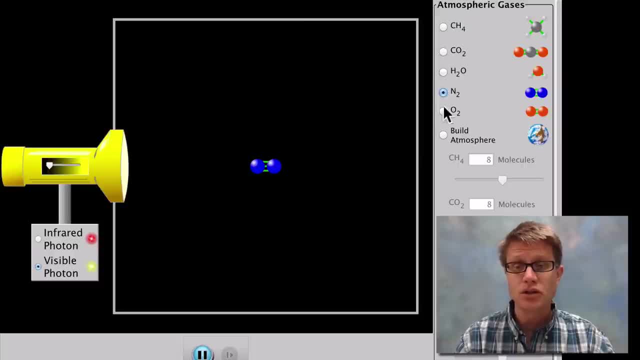 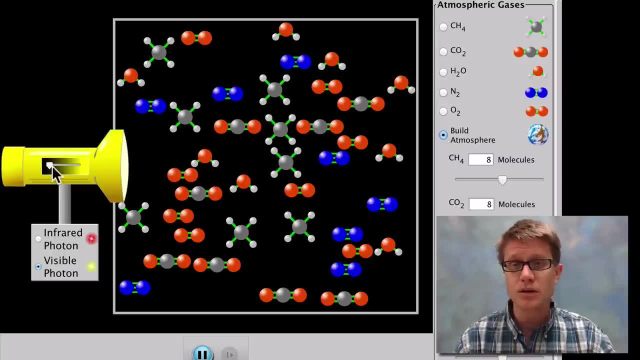 We've got carbon dioxide, water vapor, nitrogen and oxygen, So let me throw all of those into just a fake atmosphere. On the left side, we've got an emitter that is going to give off either visible radiation light- we'll call that- or infrared radiation, And so what do you? 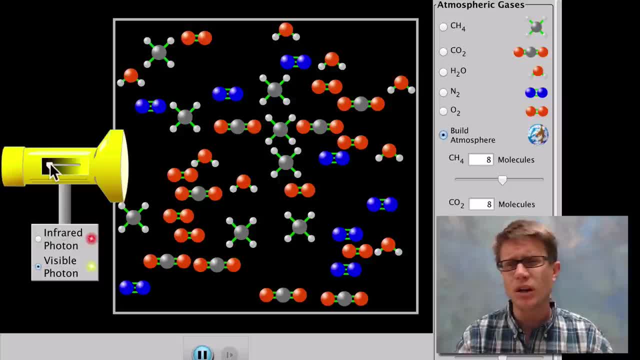 think is going to happen when we hit these all with light. Assume that molecules can't move around. Well, if you watch this as the light moves through it, nothing happens. In other words, it's not affecting those molecules at all. Okay, So what happens if we turn off light and then we turn on infrared light? So this is going. 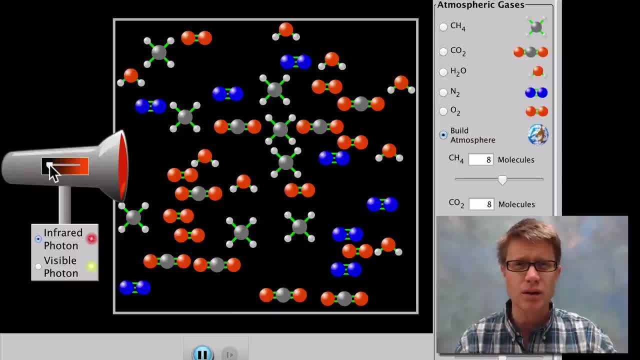 to be infrared photons. You should make predictions about what you think is going to happen. So let's turn this on now, So you can see that some of that heat is being bent and refracted and it's actually coming back from where it was. Can you see a pattern of what molecules? 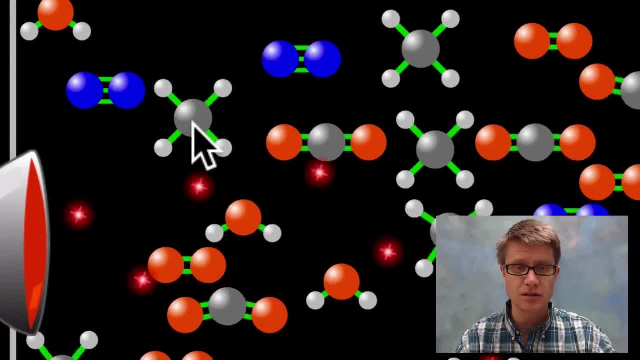 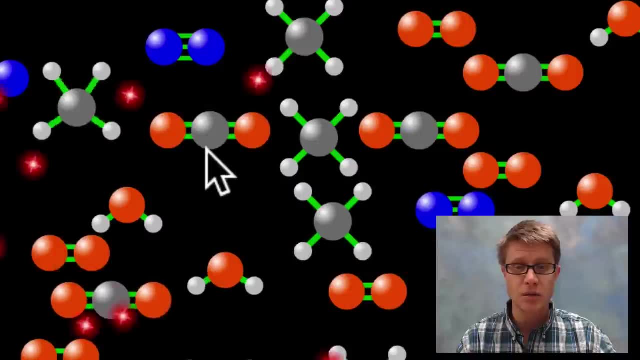 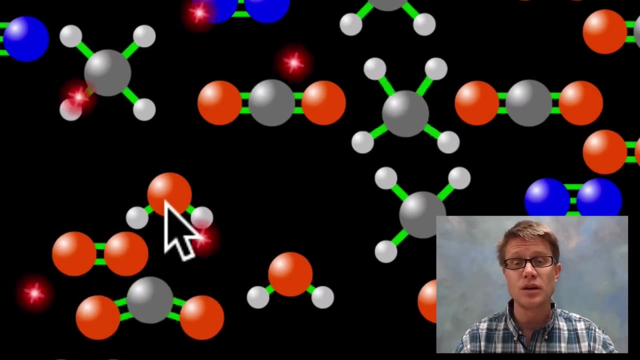 are vibrating. So let's see, I see methane is definitely vibrating right here. What else do we see? So there's another methane. I see carbon dioxide. So a carbon dioxide right here is moving. And what's the other big one that's moving? That would be water. So the water is vibrating and re-emitting. 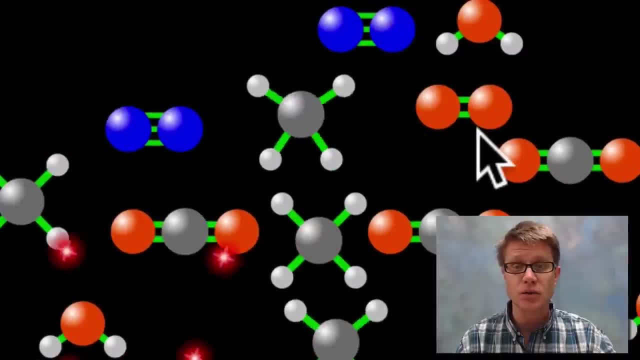 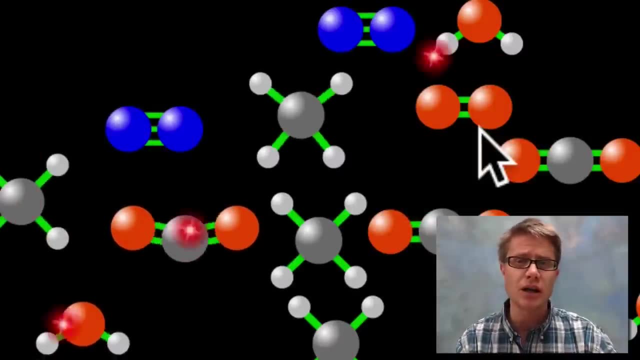 that heat? If you look at things like nitrogen gas or oxygen gas, they're unaffected by heat. And so what does that tell us? Well, if our atmosphere was just made up of nitrogen and oxygen, light would come in, heat would go out and we would have a really cold temperature. 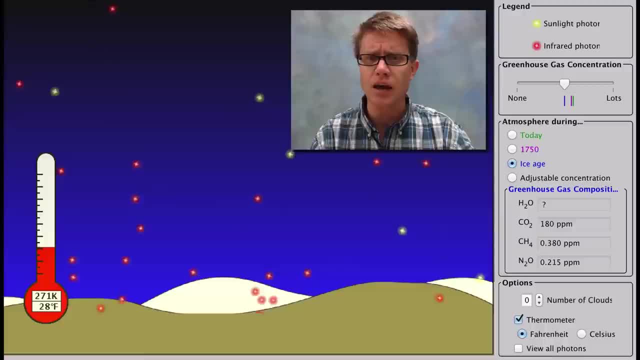 on our planet. So we need these greenhouse gases. Let's take a look at how that affects aspects, our atmosphere, At the level of the atmosphere itself, And so what I've done is turn back the clock a little bit. So we're in the last ice age. This shows our greenhouse. 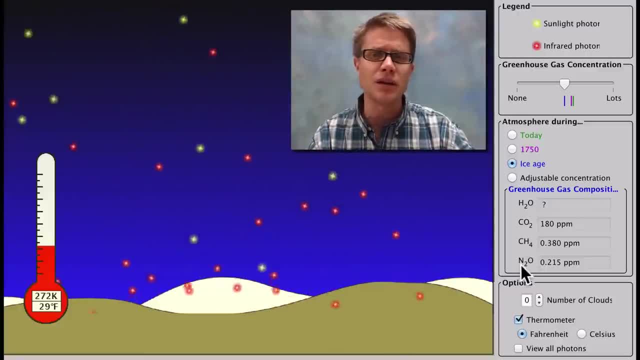 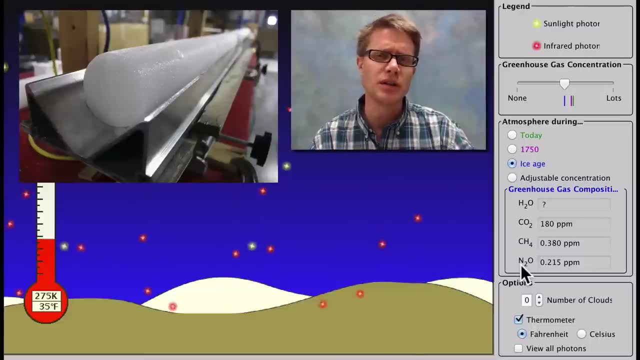 gas compositions. Now, this is thousands of years ago, And so you might think like, who was keeping track of greenhouse gases at that point? Well, nobody. If we look at ice cores, what you'll see is there are layers in the ice cores Where we had summer, winter, summer. 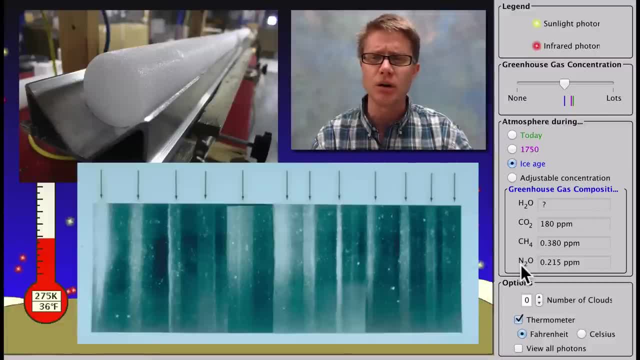 winter, summer, winter, And so you can count back and figure out how long ago it was. And then little bubbles of the atmosphere are trapped in the ice. So we can take out a section, We can add it to a mass spectrometer And we can figure out what's the composition. 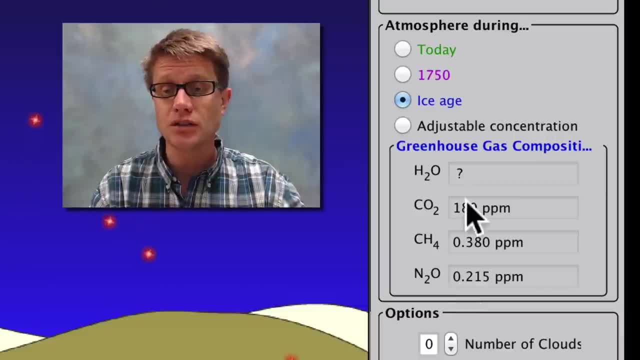 So we can see how much carbon dioxide, methane or dinitrogen oxide- These are all greenhouse gases- Water actually we don't know, because I mean, the ice is water, But we can figure out what the composition was back then, And so what did it look like back then? We had 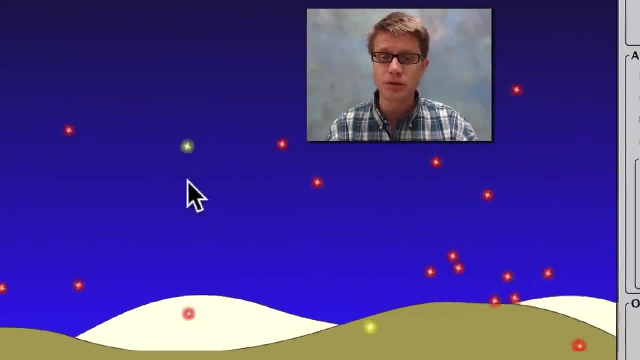 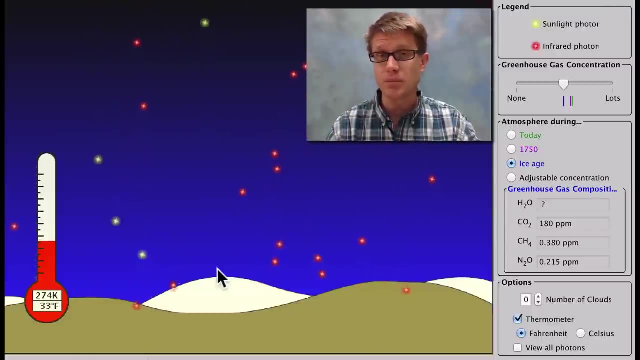 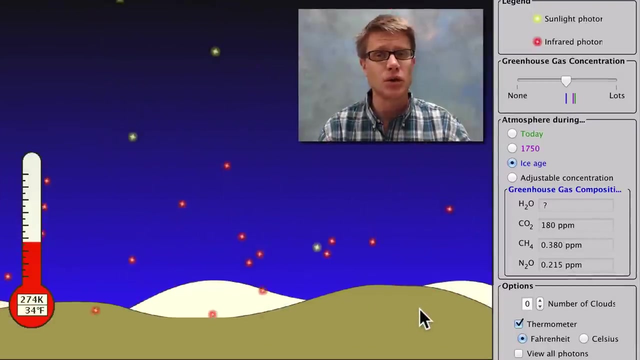 a lot more ice for sure, And so watch what happens: as a visible photon hits the ice, It just bounces right back again, And so as visible photons hit the ice, it's reflected back into space, So we're not getting that heat energy. If you look at photons then that are hitting the soil- they're being converted. 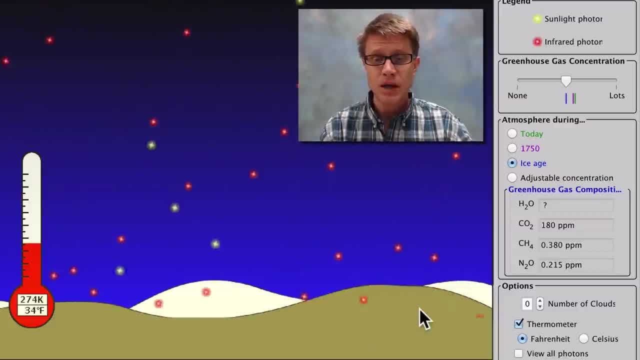 into infrared photons, and so we think of that as heat. And so as they move up, they're doing this kind of crazy dance: Some of them get refracted, Some of them get bent back towards the atmosphere and some eventually move off into heat. But since we have a low level of 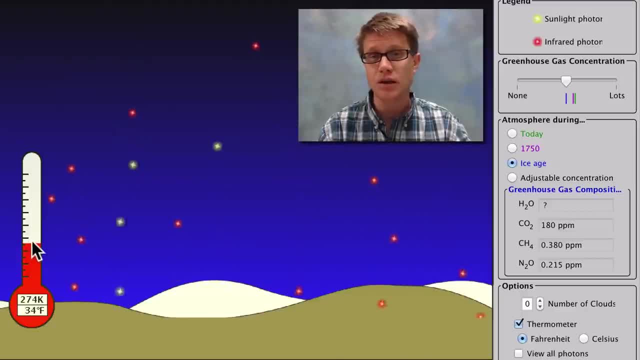 these greenhouse gases. we're not holding much of them to the planet, And so this area. we would have a temperature of around nine degrees Fahrenheit And we're going back a 34 degrees Fahrenheit. Let's move forward a little bit. So take a look at these greenhouse. 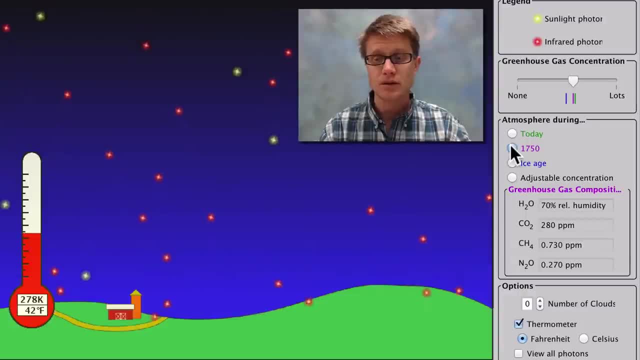 gas compositions. I'm going to move forward to 1750.. And so what do we see then? Higher amounts of greenhouse gases. So these were actually recorded by people, So we have higher amounts. So what are we seeing now is an increase in temperature. What's causing that? We're 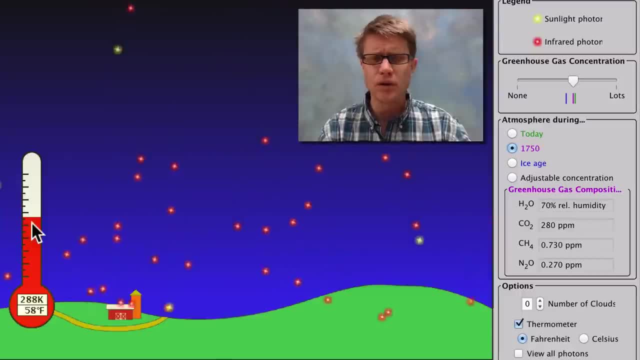 holding more of that heat close to the planet. What happened when we got rid of all that ice? More of that light, instead of being bent back into space, is actually being absorbed as heat. It's normal to see changes in the greenhouse gases, But let's look as we move. 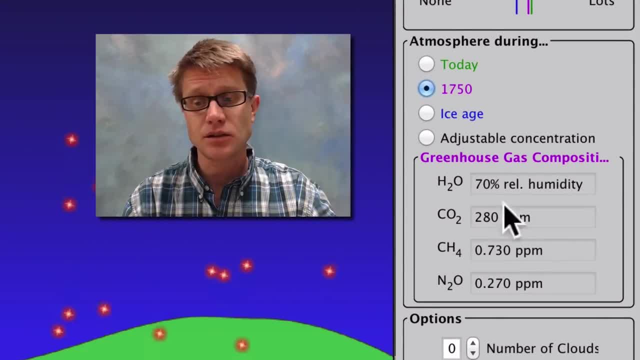 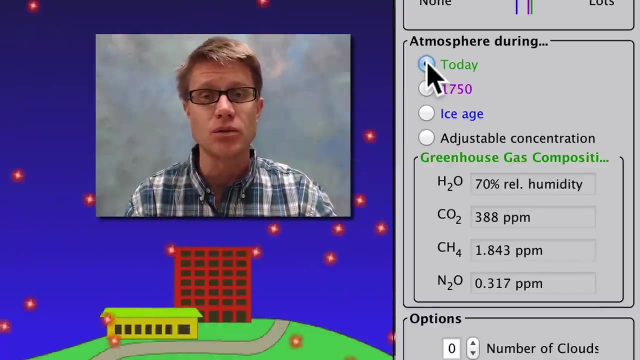 forward from 1750 until today And so especially look at these numbers right down here As we move forward. So we see huge increases in those greenhouse gases. Again, if we go from carbon dioxide, it was 280.. I just checked today It's well over 390.. I think 397.. We're 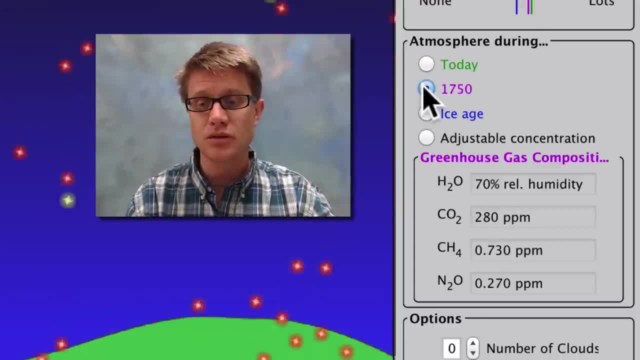 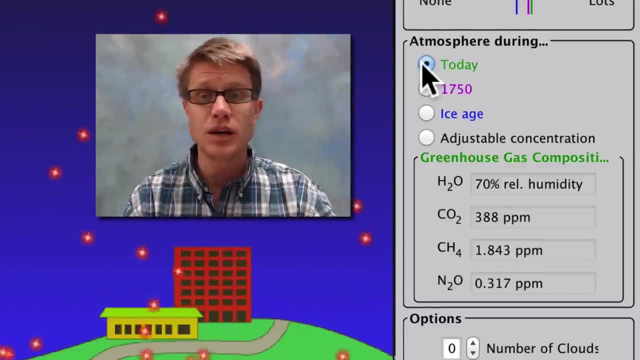 pushing 400 parts per million. We're seeing huge increases in the other greenhouse gases- If you look at methane, for example- And so what's happening? Well, the greenhouse gases are going to be very, very, very high, And what's happening with that is we're seeing 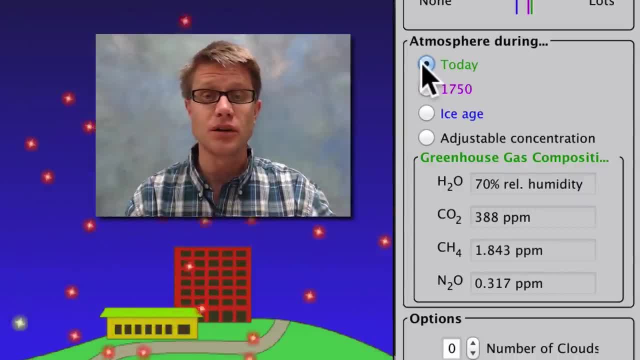 increase in the greenhouse effect, And a lot of this is caused by greenhouse gases that we're putting into the atmosphere, And so the industrialization is really increased amount of those greenhouse gases And what we start to get is a greenhouse that kind of builds on itself. Let me talk about two ways that that occurs. So, for example, if we 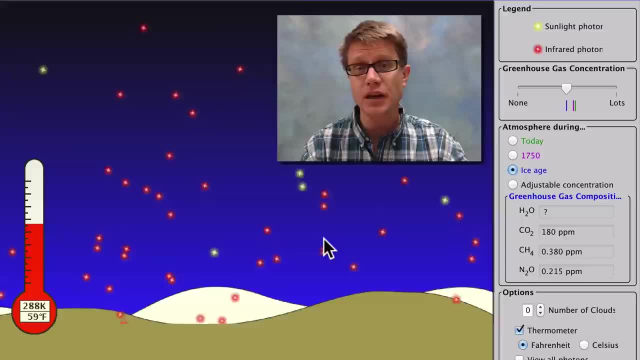 go back to the ice age. what happens as we start to melt the ice on our planet? Well, as we melt the ice on our planet, then there's more light being absorbed by the planet And heat. Another thing that happens up in the north that as we heat the permafrost it releases.